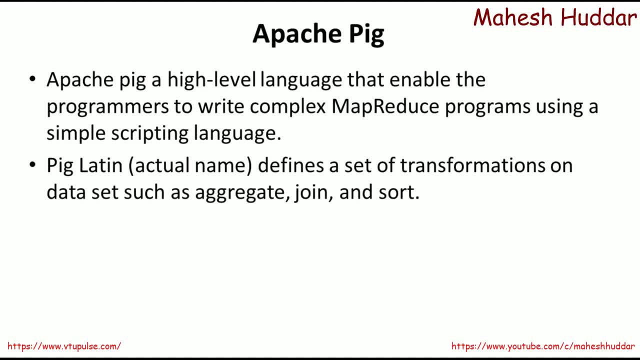 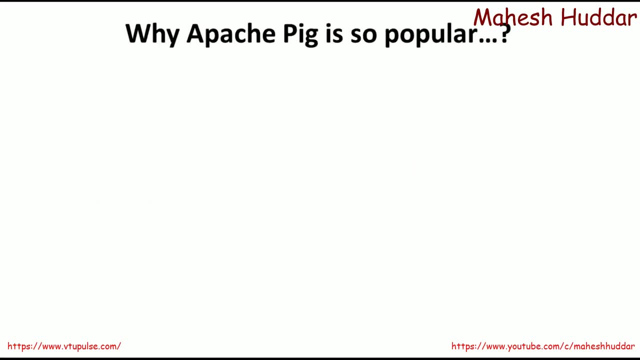 So, rather than writing a complex code for doing all these things, we have very simple commands in Apache Pig. Using that, we will be able to implement all these things easily in Apache Pig. It's an open source platform developed by Yahoo. Now why Apache Pig is so popular. 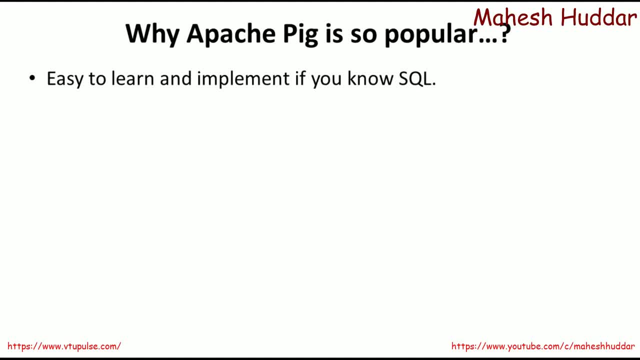 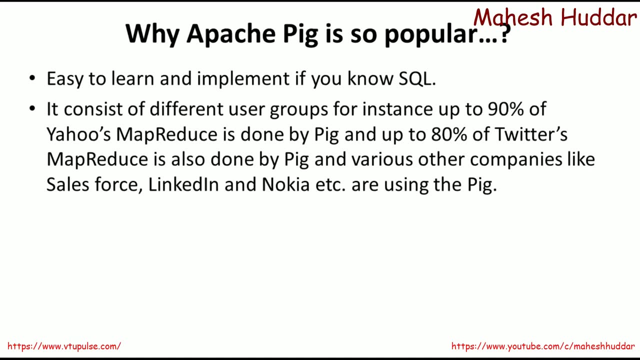 The very first reason is if one knows the SQL he can easily learn and implement the Apache Pig. That is a very important thing about Apache Pig. The second thing is many of the companies- if you go with Yahoo, all its MapReduce programs are done in Apache Pig. 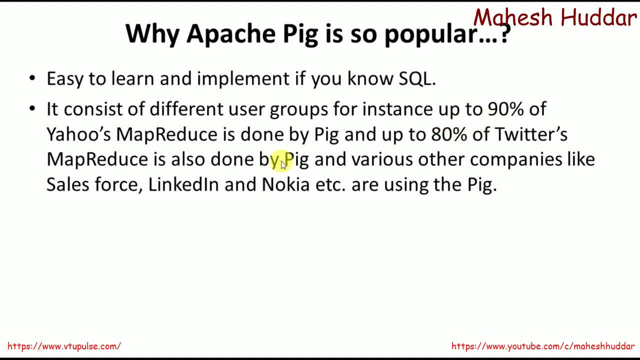 Almost 90% of the programs are implemented in Apache Pig, And various other companies like Salesforce, LinkedIn and Nokia are using Apache Pig to implement MapReduce programs. Apache Pig provides support for both scalar as well as a large number of nested and nested or complex data types. 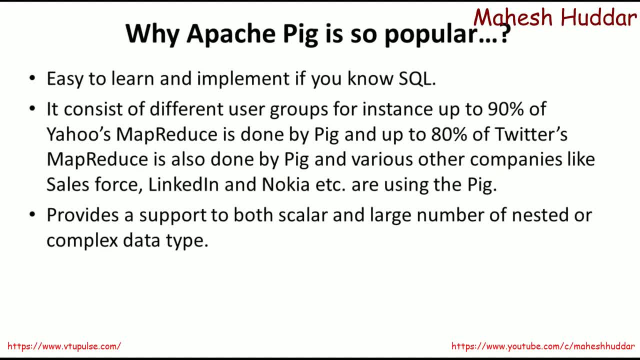 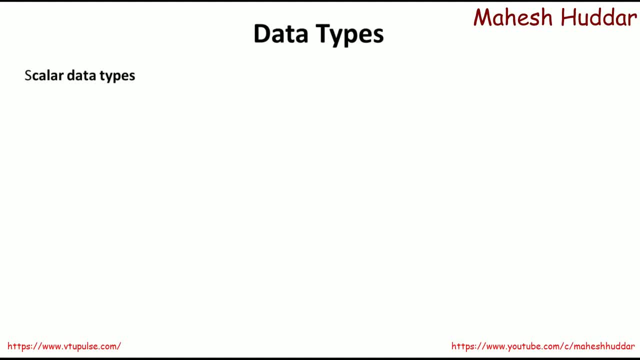 So first we'll see what are the different data types it supports and later we will see what are the modes in which it can work in Apache Pig. So the scalar data types are: int, float, double long char array. 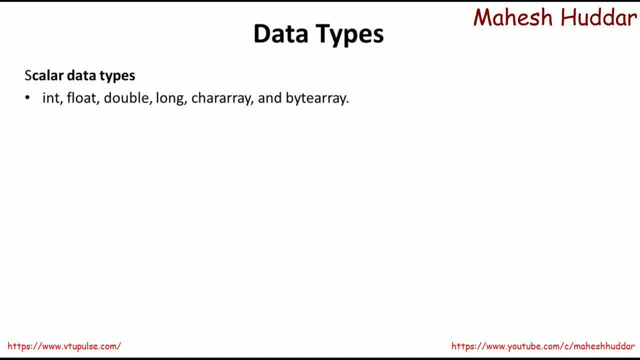 So the scalar data types are: int, float, double long char array. These are all the scalar data types Apache Pig provides And it supports complex data types. This is a very important thing. in Apache Pig There are three complex data types. 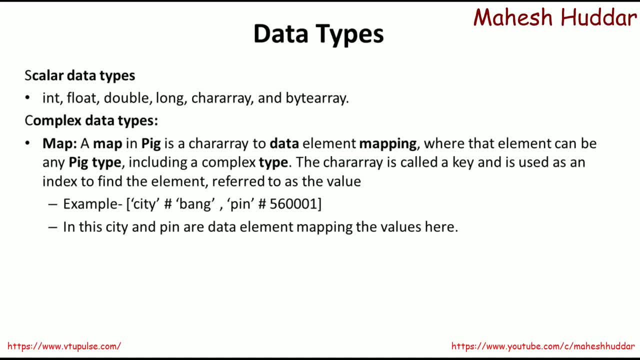 The first one is map. It is like a dictionary in other programming languages, where we have a key which is used to index the values. The values can be of any pig data types. It may be a simple or it may be a complex. So in this case, city is a key and b a n g is a value, p? i n is a key and 5,, 6,, 0,, 0,, 0,, 1 is a value. 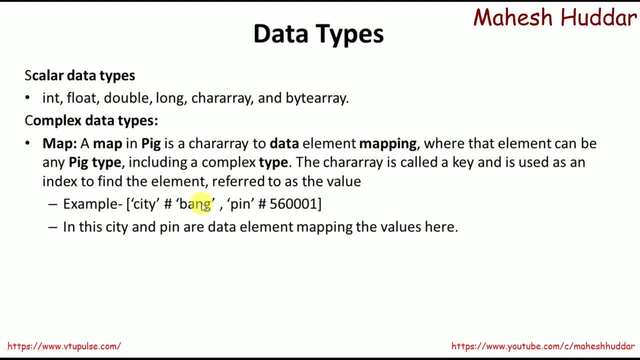 So this is how actually we can create a mapping between keys and values in Apache Pig. The one thing is, the values can be of any type. It may be a scalar data type or it may be a complex data type. So that is the very important part here. 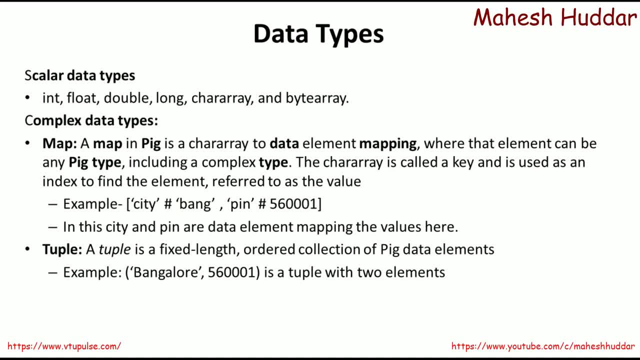 The second complex data type is tuple. Tuple is a fixed length, ordered collection of pig data elements. So it's a length. So it's a fixed length, ordered collection of pig data elements. So it's a length is fixed Once it is defined. we cannot alter that particular length and it's an ordered collection of pig data elements. 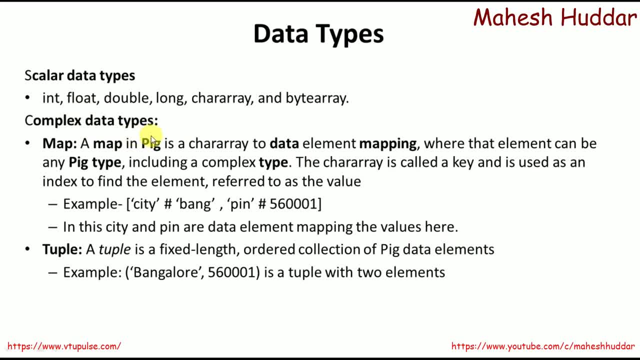 So what are the pig data elements we have? It may be a scalar or complex data elements. It's a collection of those particular data elements and once it is defined, it cannot be altered. So in this case, if you see, it's a tuple with two elements and each of these elements are separated by comma. in this case, 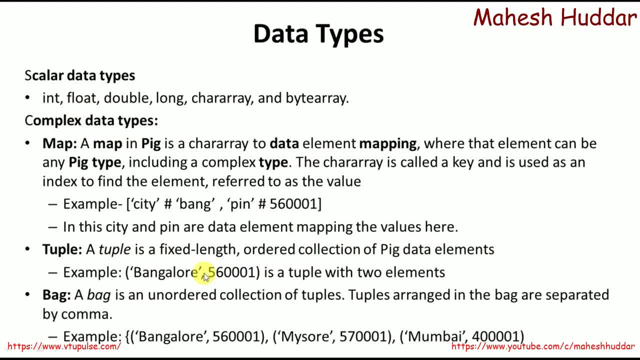 So this is how we can create a tuples. The last one is bag. Bag is an unordered collection of tuples. So it's a collection of tuples, and these tuples are not necessary that they should be in an ordered fashion or something. It's an unordered collection of tuples. 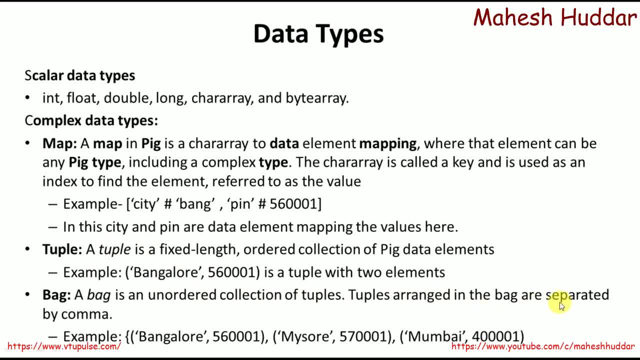 And each of these particular tuples are arranged in bag by separating, separated by comma. For example, this is one tuple and the second tuple and third tuple. This is a bag consisting of three tuples and each of them are separated by comma, in this case. 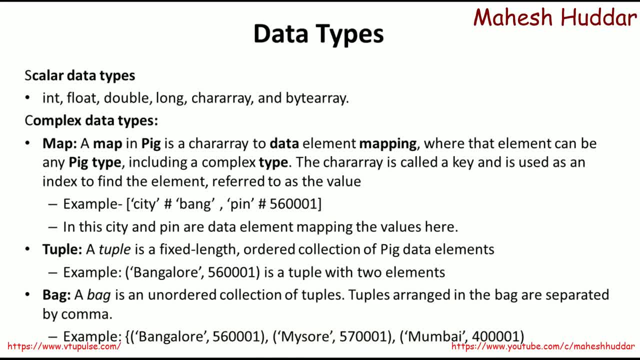 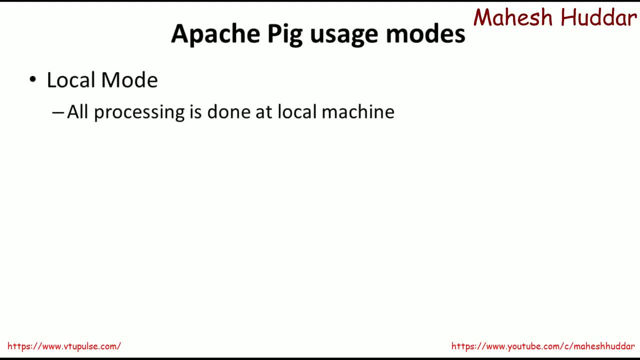 So this is how actually we can have the complex data types in Apache Pig. Now, what are the modes in which we can use Apache Pig? So we can use Apache Pig in local mode. All the processing is done at the local machine. 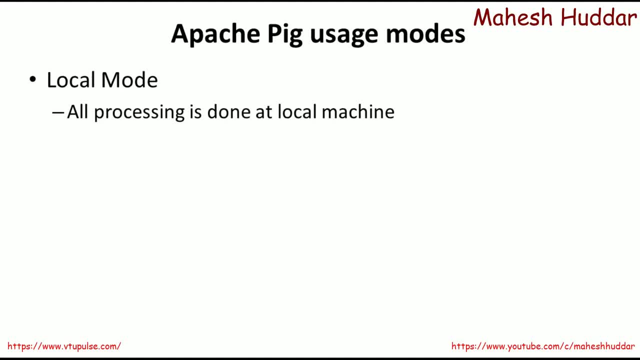 There is nothing called as HDFS or cluster of machines or anything. Everything is executed on local machine. We can install it on a local machine and then run our scripts on a local machine. The second one is non-local mode, or you can say that the cluster mode. 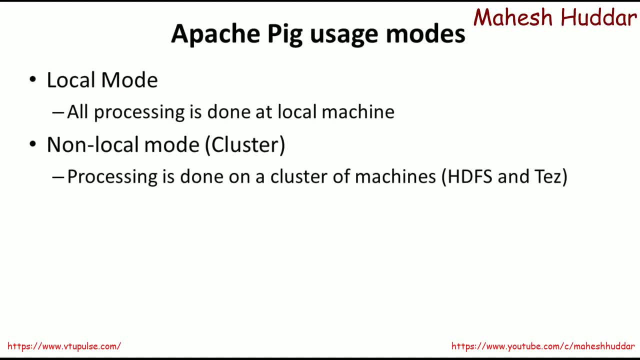 The processing is done on a cluster of machines. So we can put our data into a cluster And then we can run our Apache Pig program on a cluster of machines. So that's another way of using Apache Pig. The third one is called as iterative or batch mode. 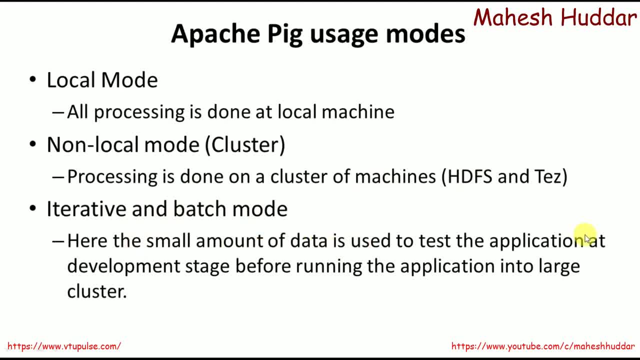 What is this is Here a small amount of data is used to test the application at the development stage before running the application into a large cluster. So before you use the whatever the program you have written in Apache Pig, rather than directly using it on a cluster of machines. 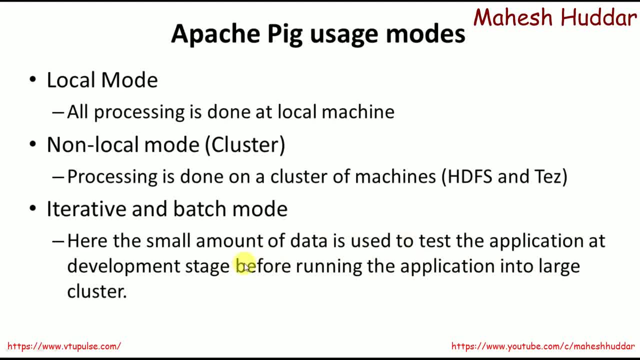 first test it with a very small amount of data. So if you run Apache Pig on a local machine, if it is working fine on a local machine with a small amount of data, then we can deploy that thing into a large cluster with a large data set. 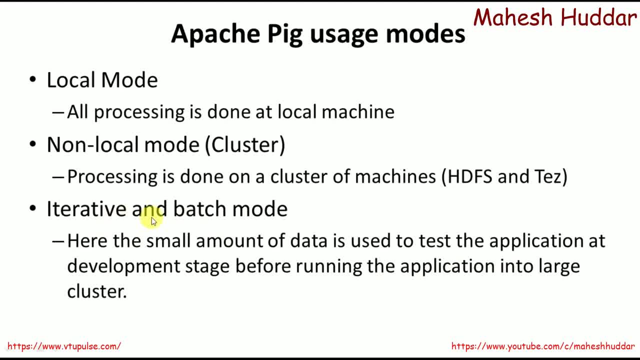 So that is what the third one You can say, it's a testing mode or something like that. So that is how actually we can use Apache Pig. So Apache Pig can be used in three modes: On a local mode, non-local mode, or you can say that the cluster. 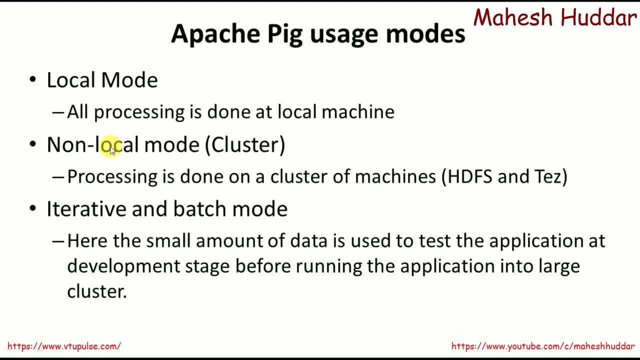 The third one is iterative or a batch mode. The next thing is how to run Apache Pig programs. So if you run Apache Pig on a local machine, you can run Apache Pig on a local machine. So if you want to run Apache Pig programs, 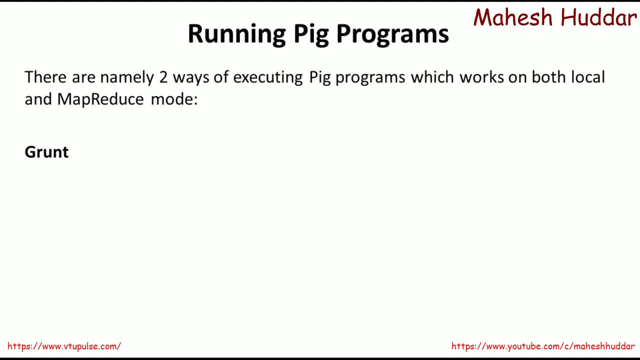 there are two methods. One thing is, we can use the grunt shell. And what is the grunt shell? It is like an interactive shell programming, where we can start typing the commands and then we can do our tasks. So this is a shell, like a unique shell or something. 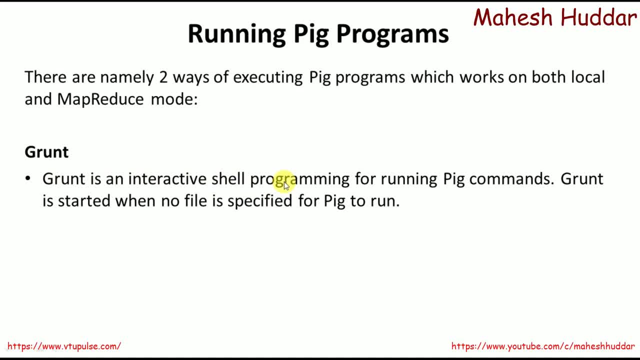 So once you get this particular shell, you just go on typing your commands which are necessary for your applications. So that is how actually we can use grunt shell. The second one is what We can put all those particular commands we want to execute into a file. 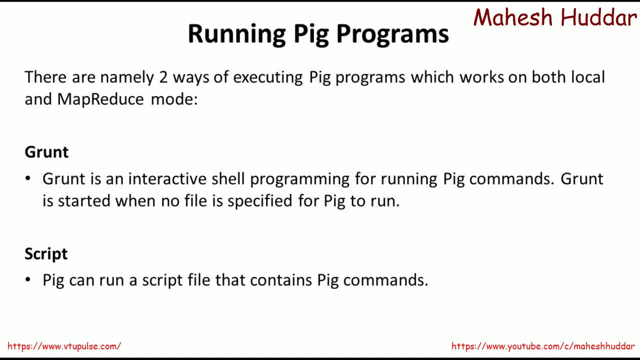 and name that particular file with some name, and the extension should be PIG in that case. So once you put all your commands into a file, you can run that particular file with the help of PIG command. That is PIG, the name of that particular file, dot PIG. 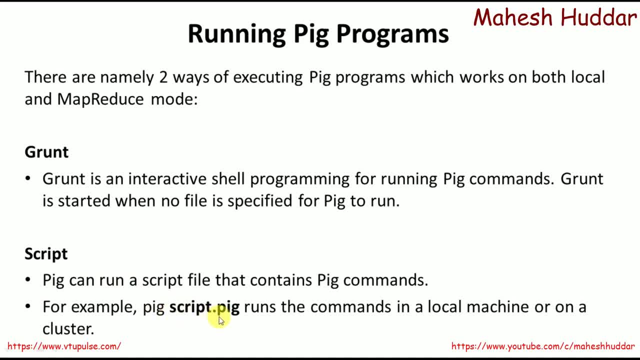 So PIG is the command and this is the name of that particular file with extension PIG. So this is how we can execute Pig commands or Pig programs. One is on grunt shell, another one is put all the particular thing into a file. 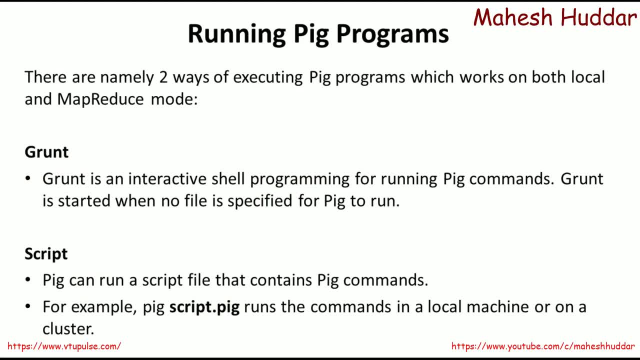 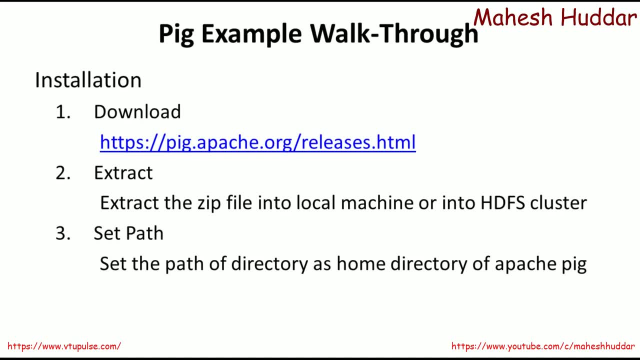 and we can say that particular file as a script. So something like that, we can run the program. Now we will take one very simple example to understand how to install Apache PIG and then run a very simple program. So if you want to install the Apache PIG, 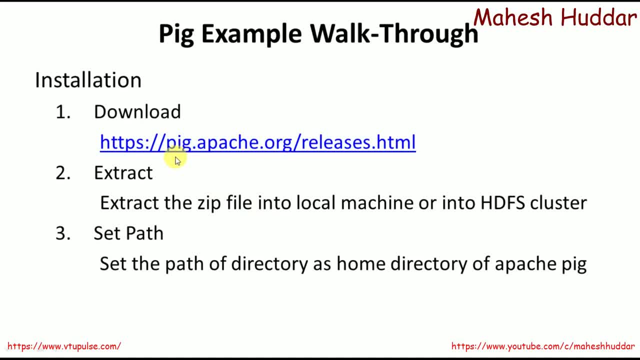 it is a very easy procedure. Only thing is we need to go to this particular website and download the latest version of Apache PIG. You will get that particular file in the form of a zip that is compressed file. We need to extract that particular zip file into a local machine. 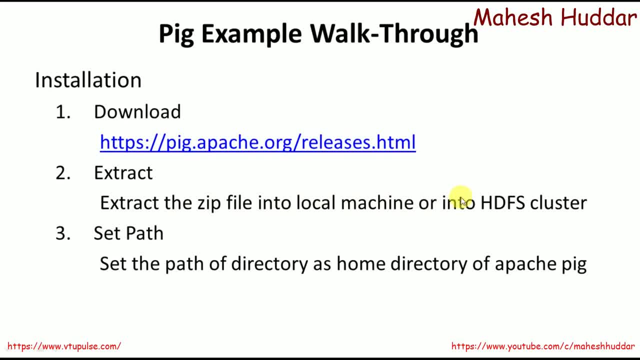 if you want to run it on a local machine or if you want to run your application in HDFS cluster, you need to extract it into HDFS cluster. Now what we need to do is we need to set the path, that is, you have extracted that particular PIG. 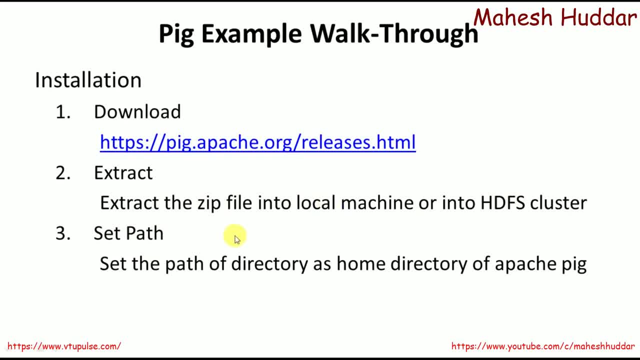 But where that particular thing is there, we need to say to our programs: because if you want to execute a program we need that PIG command. So we need to set that particular directory where you have extracted that particular PIG as a home directory for Apache PIG. 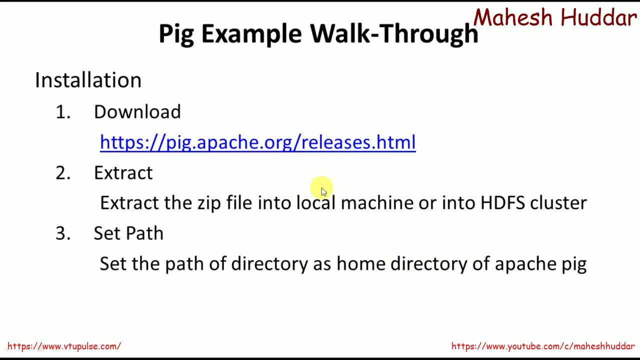 So once you set that particular directory as a home directory, you will be able to run your programs. So this is the very simple way of installing Apache PIG. First, download it. extract that particular zip file on a local mode or in a HDFS cluster. 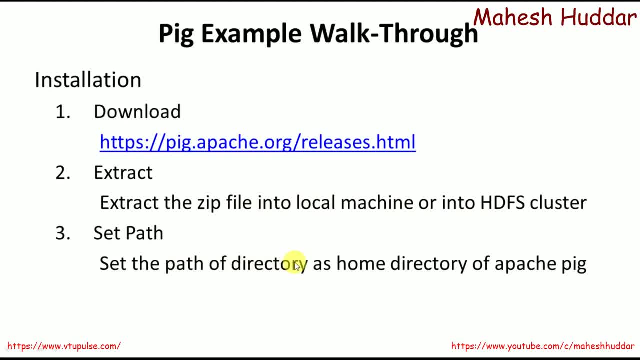 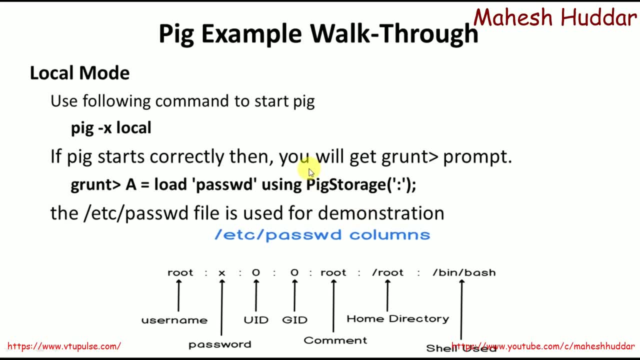 set the path of the directory where you extracted the data as a home directory for Apache PIG. So once you have downloaded and installed Apache PIG, the next thing is to run a very simple example. So if you want to run a program, 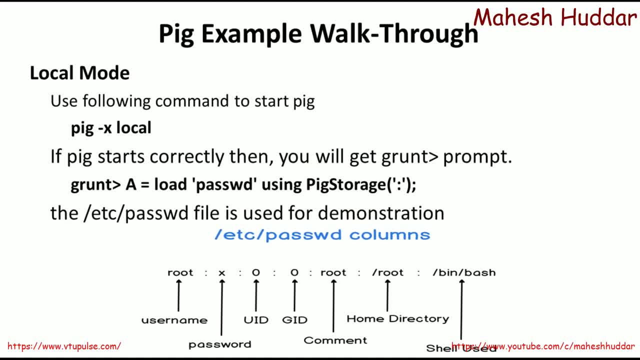 you can run it on a local mode or you can run it on a cluster mode also. So if you want to run your program on a local mode, we need to use this command, that is, pig-x local. So what it does is: 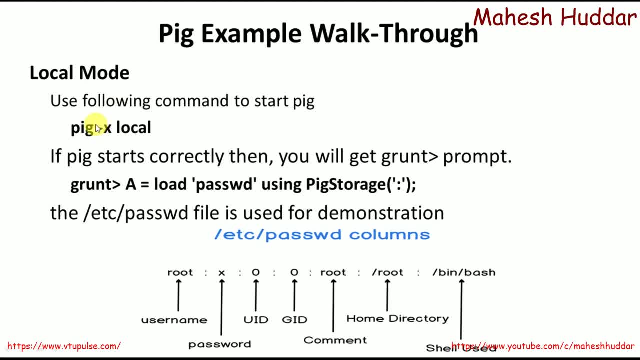 it will start an interactive shell, or you can create a script also so that you can run that particular thing. So first, once you type this particular program, a grunt shell or a grunt prompt will be opened to you. That is something like this: 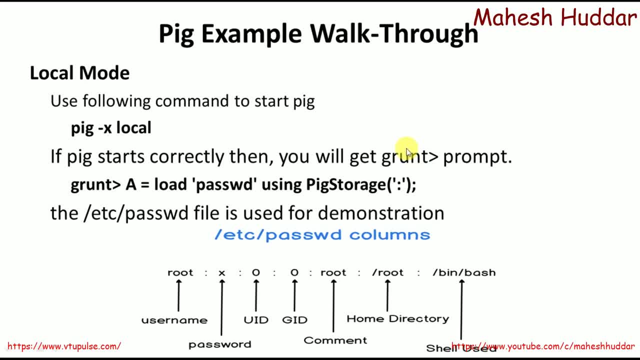 On the top of it you can write your commands. So before I go through the commands and all, to demonstrate this particular example, I have taken a very simple file. The file is etc. slash, passwd. So what it contains is: 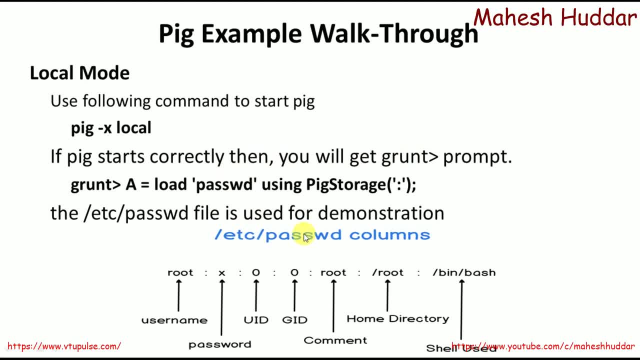 it contains the information or the user name, user information who are working on a particular Unix machine. It contains different fields like username, password, UID, GID and so on. This is the file I will be taking as an input so that I can extract some of the fields from this particular file. 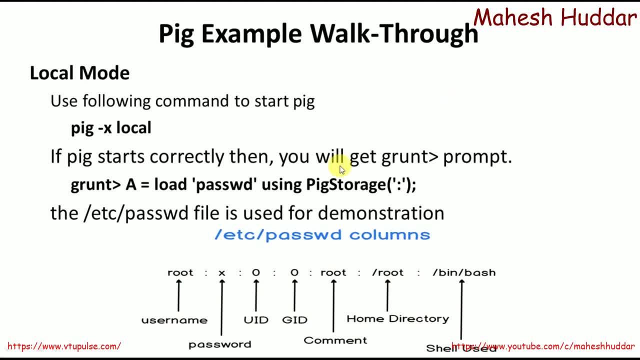 So that is what the thing Now, once you get this, once you run this particular command, you will be getting a grunt prompt. Now you can start writing your command. So if you want to load this particular file, the very simple command is what: 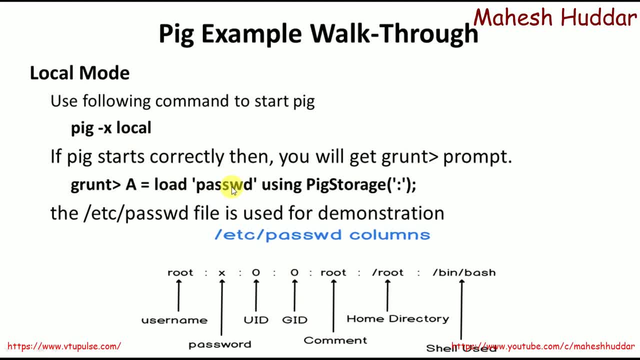 Load, passwd. That is, load is the command. passwd is the file name. Using what Pig storage? I want to use pig storage in this case and then I want to load this particular file. But when you want to load this file, 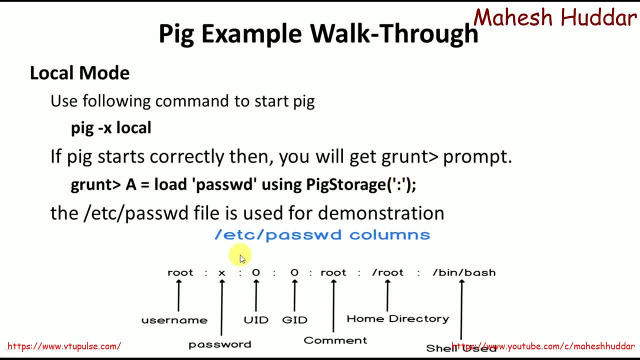 there is one thing we need to mention: What is the delimiter for each and every field? If you look at this particular file, the delimiter in this case is colon. in this case, Sometimes it may be space, sometimes it may be tab or whatever it may be. 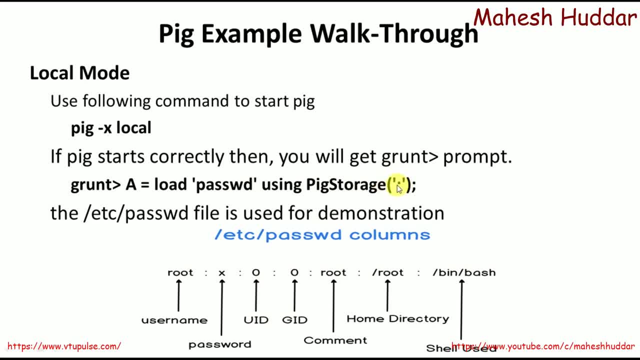 Depending on your file, we need to pass the delimiter in this case. So, depending on the delimiter, each and every line and fields of this particular file will be loaded into A here Now, once the data is available in A. so each and every row of this particular thing is present in A. 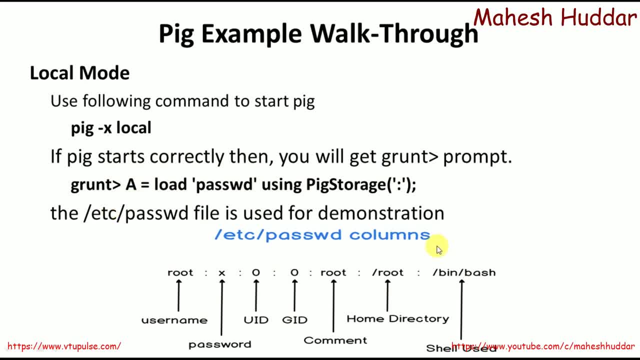 So you can read the data row by row and then, whichever the field you are interested- For example, you may be interested in username, or you may be interested in comment, or you may be interested in shell used- So you can get that particular field. 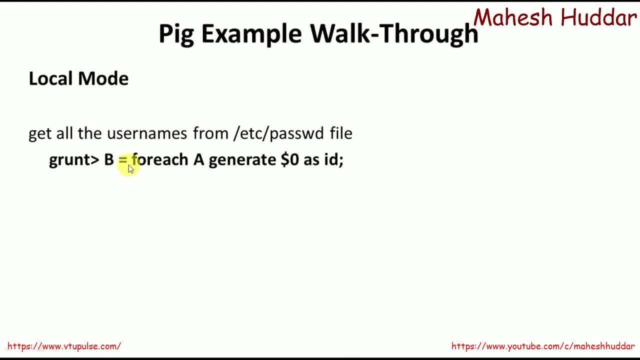 So how can you do that? one is, you can use this command, That is, for each A, that is for each row in A in that particular file, generate $0 as ID. So if you look at this particular thing, $0 is nothing but what. 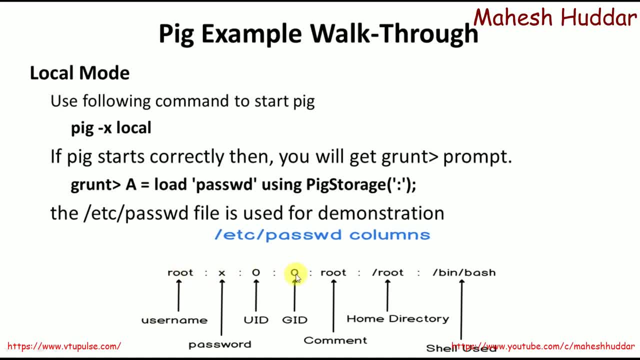 $0 is nothing but the first field: $1, $2,, $3, $4.. $5, $6.. So this is how these particular fields will be recognized. So I want username. So it is presented where. 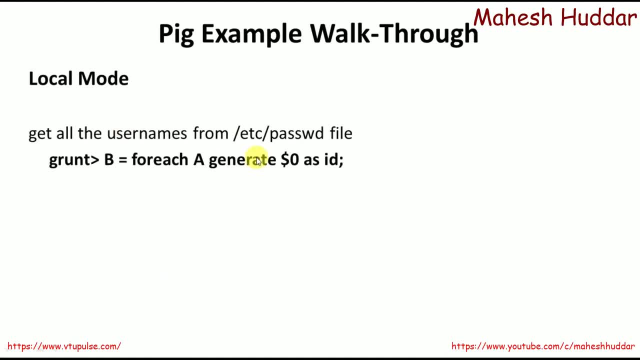 It is presented $0.. So what we need to do is generate $0 as ID. So it is a variable and it is the place where that particular data has to be extracted and it should be put into this variable and it should be done for each and every row. 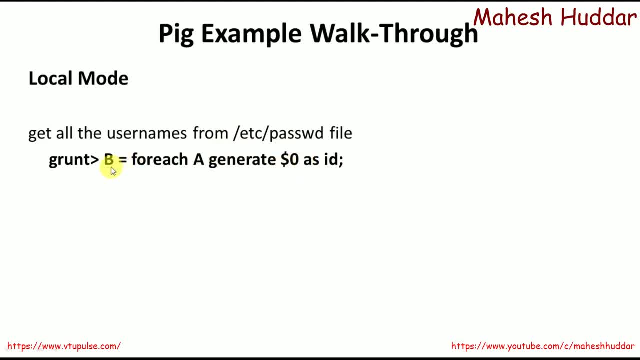 and entire information should be stored into B here, Once usernames are available, you can display those party thing with the help of dump b, So all the information you have extracted. it will be displayed onto the terminal Now, if you want to close this particular local mode. 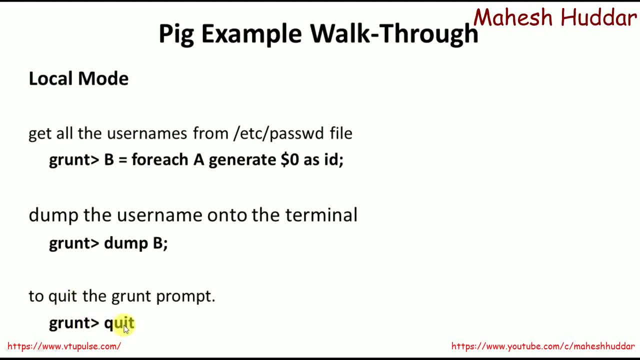 we can use grunt quit, So this is the one thing we can do. Let us say that I am interested in running a script, So what I need to do is I need to write all these particular commands into a file and then name that particular file as 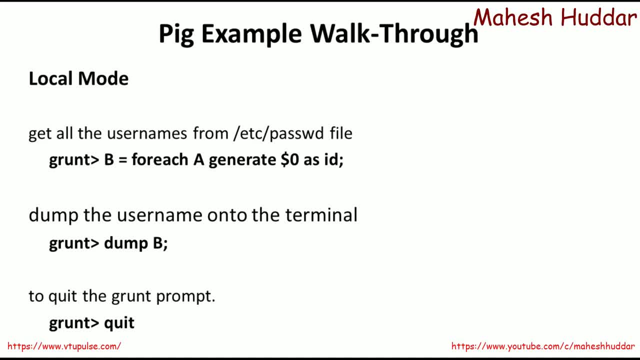 filenamepig, and you can run that particular thing on a local mode also. So how to run it? pig, that is a command space, filenamepig, something like that. we can execute it on a local mode. The same thing can be done on a cluster mode also. 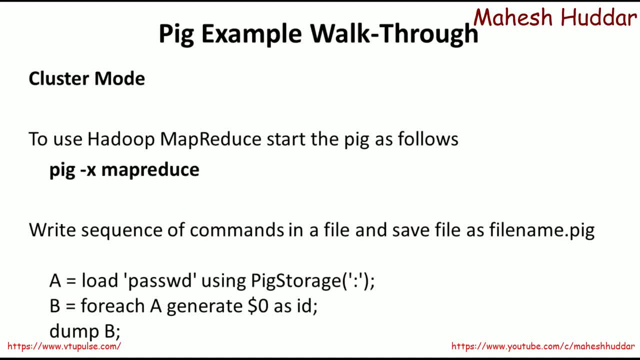 So if you want to run a pig example or a pig program on a cluster mode, the first thing what we need to do is we need to start pig in cluster mode. That is, if you want to start pig in cluster mode. 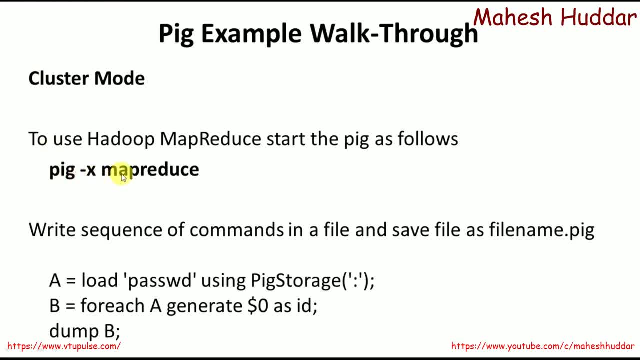 we need to use this command, That is, pig minus x. In the previous case we have used local mode there. In this case we need to use map reduce. Now the pig will start in map reduce mode If you want to run any program. 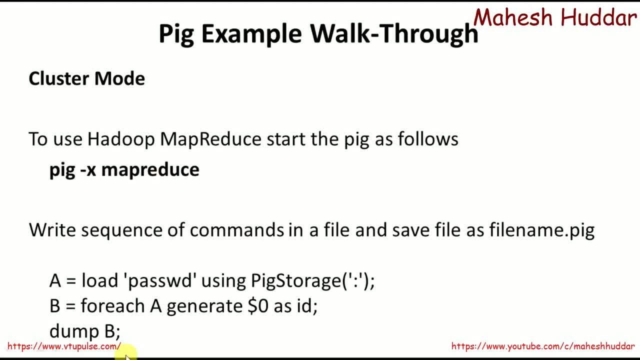 we need a script in map reduce. So first we will write a script here. So script contains three lines. What is that? First we need to load the file using pig storage into a variable. a For each line in a. 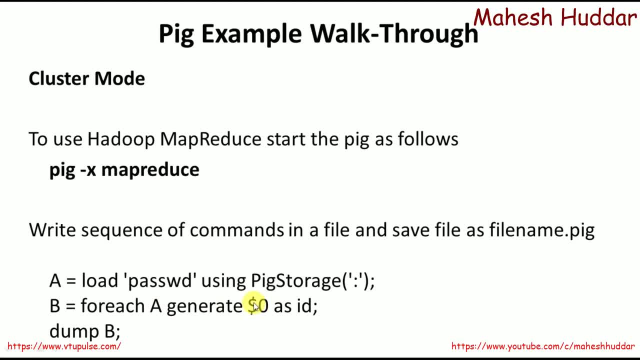 generate $0 or get the $0 element and put it into id. Once all the data is read, put entire information into b And then display that information onto the terminal. So this is what the program, The same thing we have done separately. 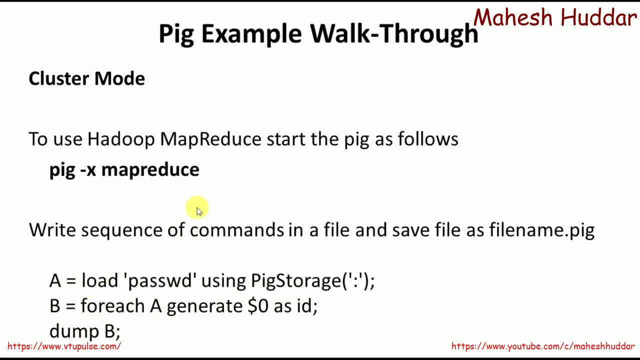 or on a grunt shell. Here we have putting all these things into a file. Let us say that the file is filenamepig. You can take any file name here. Just for example, I have taken filenamepig Now if you want to run this particular program.